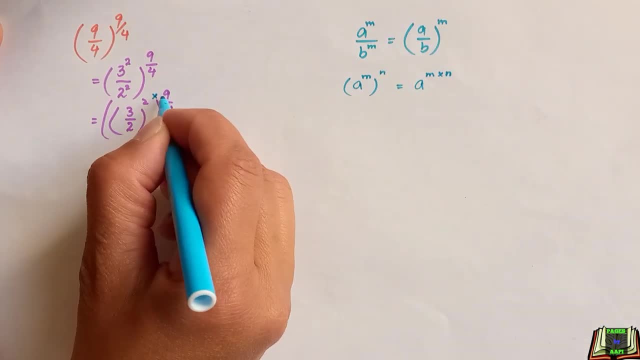 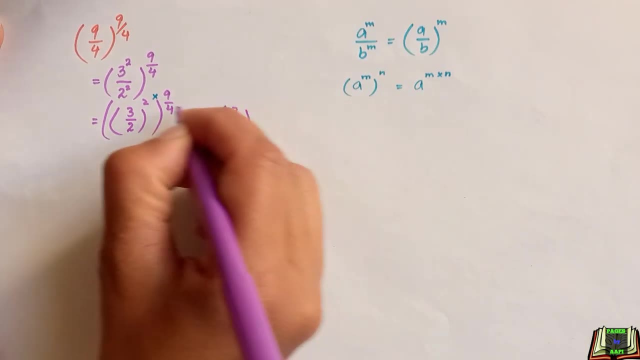 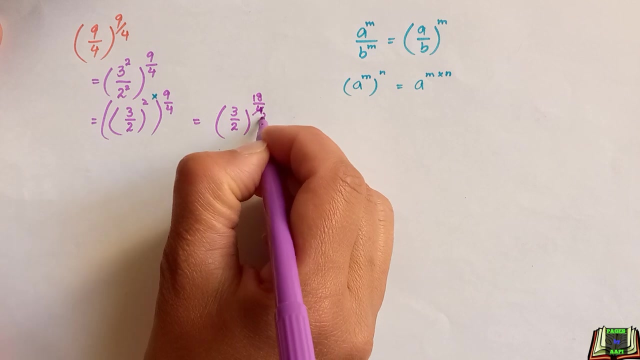 times n. So we are going to multiply these two powers and after multiplying, this is equal to 2: 9 times is 18, divided by 4.. 2 times 2 is 4 and 2, 9 times is 18.. This is equal to. 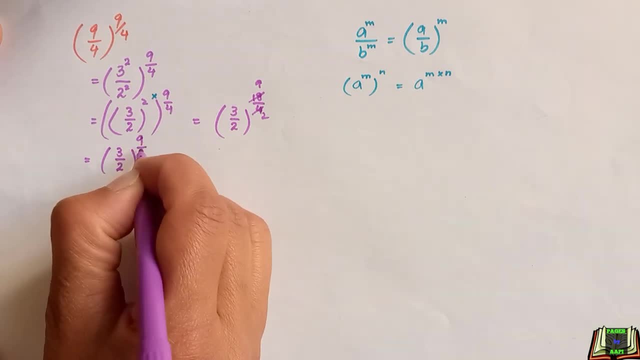 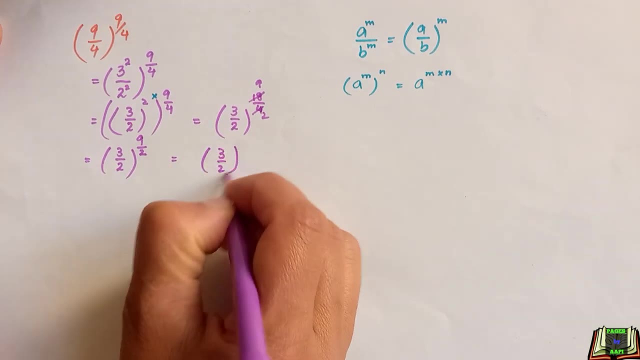 3 divided by 2 to the power 9 divided by 2.. Now writing 9 to its equivalent value, like we can write it as 3 divided by 2, 4 plus 5 divided by 2, and writing it separately this will be equal to. 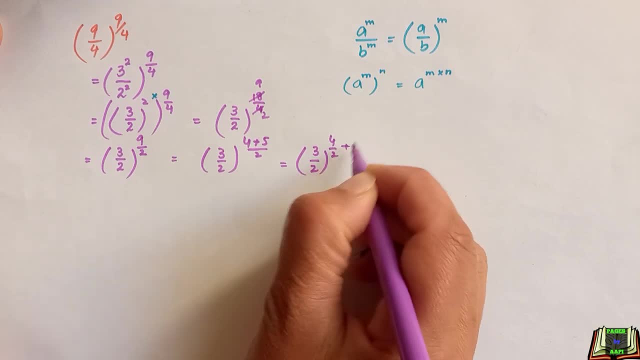 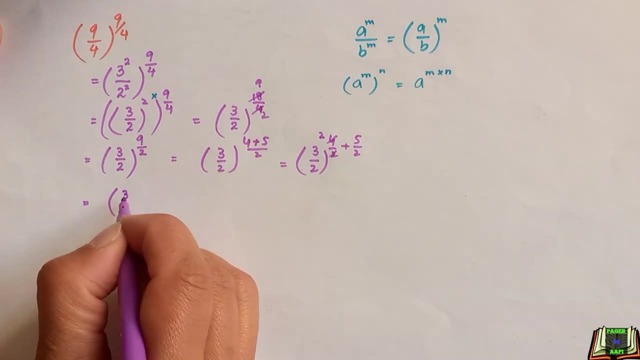 4 divided by 2 plus 5 divided by 2.. 2 times 1 is 2 and 2 times 2 is 4.. 3 divided by 2 to the power 2 plus 5 divided by 2.. Here is another power rule that says: if a 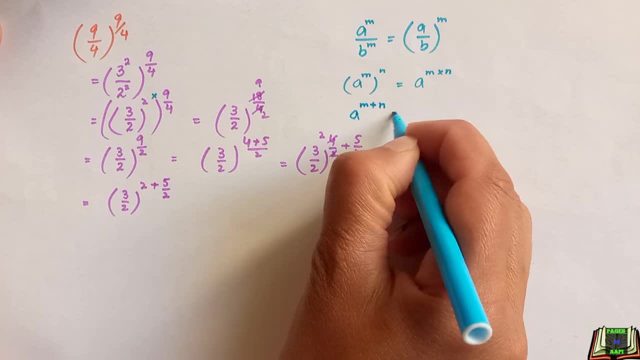 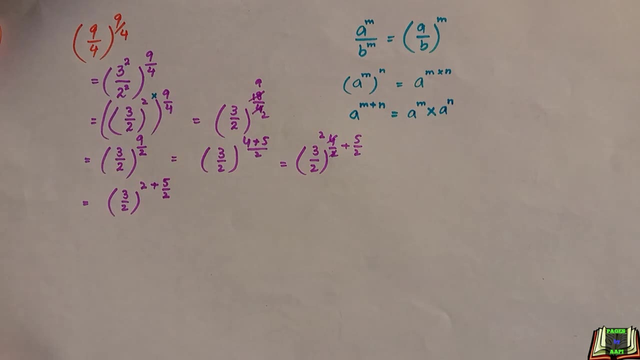 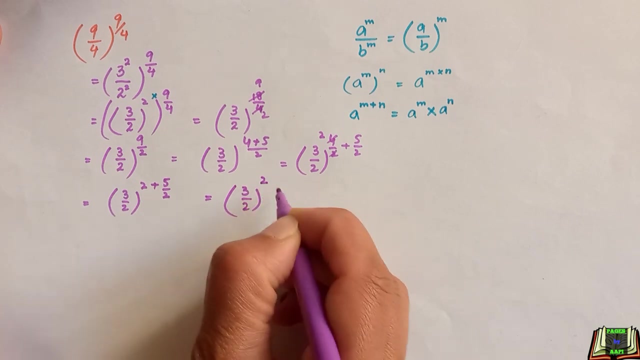 raised to power m plus n, then this is equal to a raised to power m times a raised to power n. We can write it as 3 divided by 2 to the power 2 times 3 divided by 2.. We can write it as 3 divided by 2 to the power 2 times 3 divided by 2 to the power 5 divided by 2.. 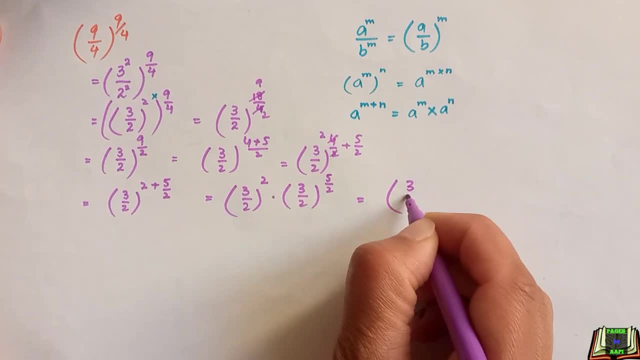 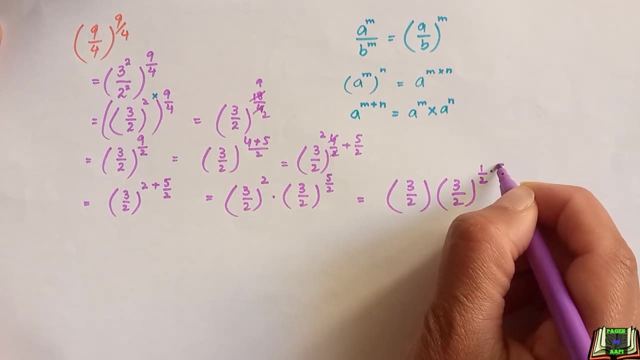 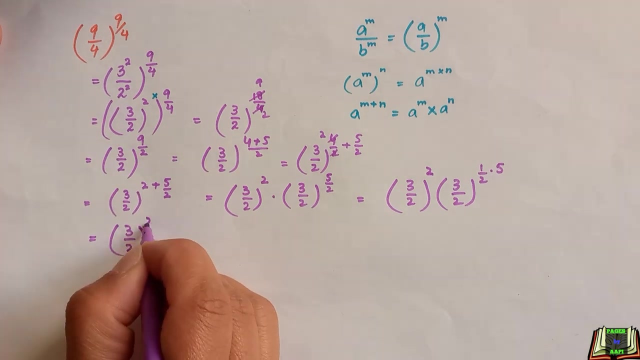 And this 5 divided by 2 is as same as 1 divided by 2 times 5.. 1 divided by 2 times 5.. 3 divided by 2 to the power 2.. Here is power 2.. And one over 2 is the value of root. So writing it in root and whole. 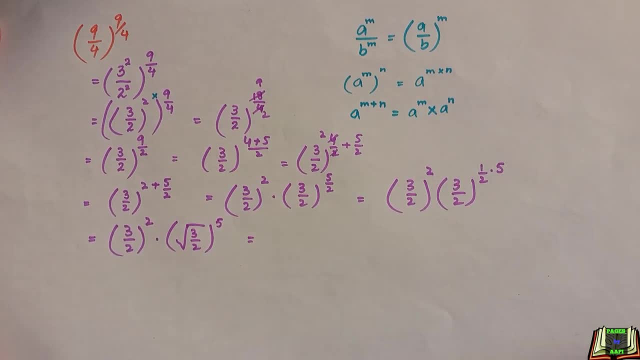 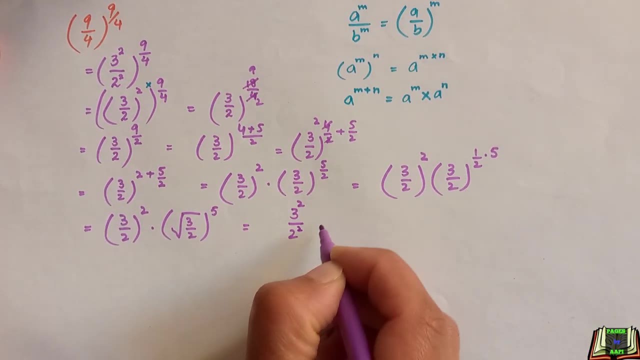 to the power 5.. Writing power separately. this is equal to 3 to the power 2 divided by 2 to the power 2 times times root 3 to the power 5 divided by root 2 to the power 5.. 3 to the power 2 is equal to 9 times. this is equal to 9 root 3. how root 3 to the power 5 means.